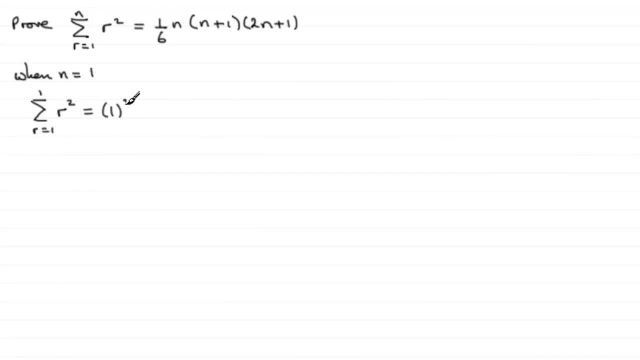 It's going to equal. It's simply 1 squared, which clearly is 1.. Now what we need to do is check out whether the right-hand side comes to 1 when we substitute 1 in for n. So we've got 1 sixth n multiplied. 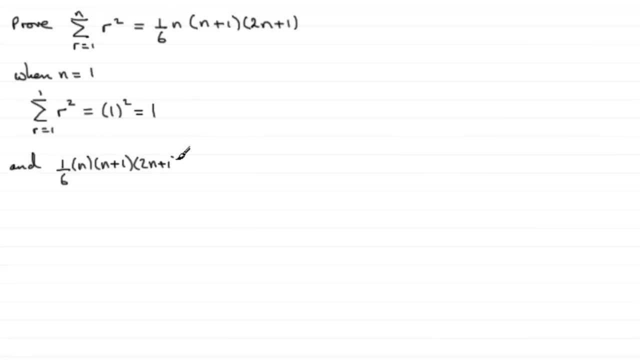 by n plus 1, multiplied by 2n plus 1.. And if we put 1 into that, we end up with 1 sixth n multiplied by 1, multiplied by 2, multiplied by 2n plus 1, multiplied by 2n plus 1 multiplied. 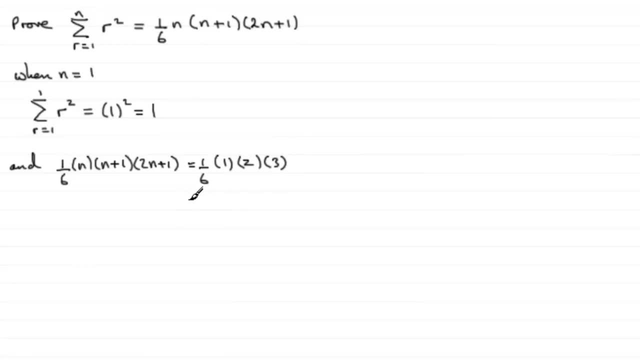 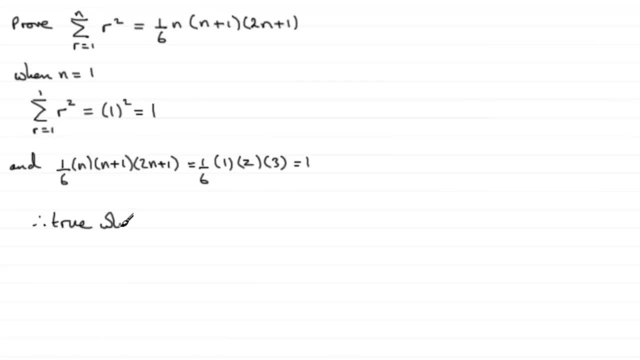 can see that it's true when n equals 1.. Now we need to assume that it's true for some particular value for n. Assume true that it's for n equals, say, k. So that means that we can say that the sum of r squared, going from 1 to k, equals one sixth, and all we need to do 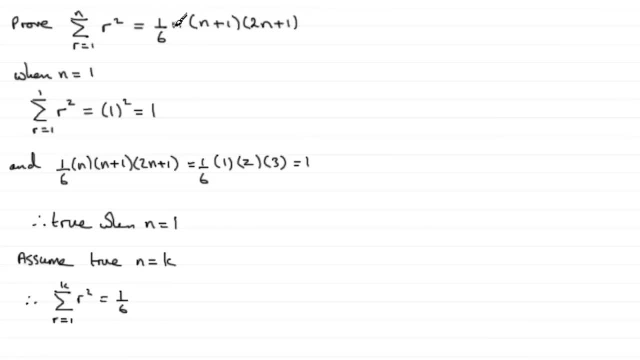 is if we're assuming this result is true for n equals k. just substitute k into here. so we've got one sixth k multiplied by k plus 1, multiplied by 2k plus 1.. Now that we've done that, we've assumed that it's true for some particular value of n. we now need to show that it's true based on this: 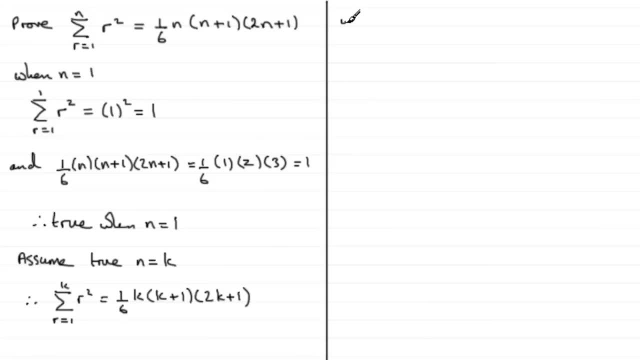 assumption for n equals k plus 1, so we'll put when n equals k plus 1.. So, when n equals k plus 1, we have the sum of r squared going from r equals 1 to k plus 1.. Now, in order to use this particular result, what we do is we say that this is exactly the same as doing the sum of r squared. 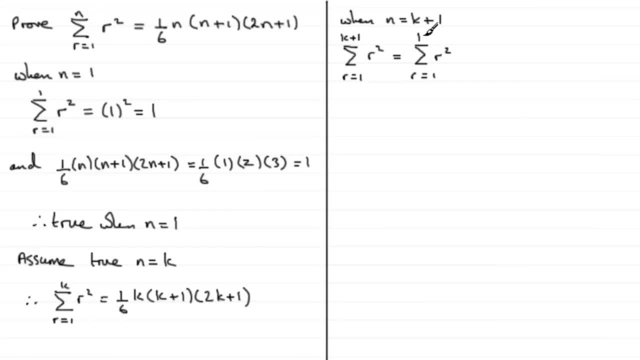 going from r equals 1 to k plus the last term, the k plus 1 term, and that would be simply k plus 1 all squared, that's when r is the k plus 1. Now we can use this result if we assume that that result is equal to this. 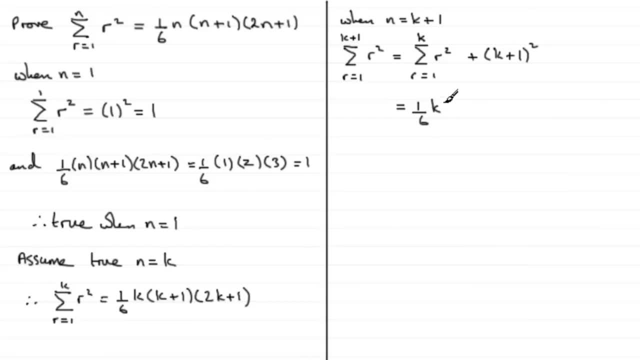 then we've got one sixth k multiplied by k plus 1, multiplied by 1.. 2k plus 1, and then we've got the plus k plus 1 all squared on the end here. Now, if we're to prove that this is true for n equals k plus 1, you would expect to see one sixth k plus 1 here. 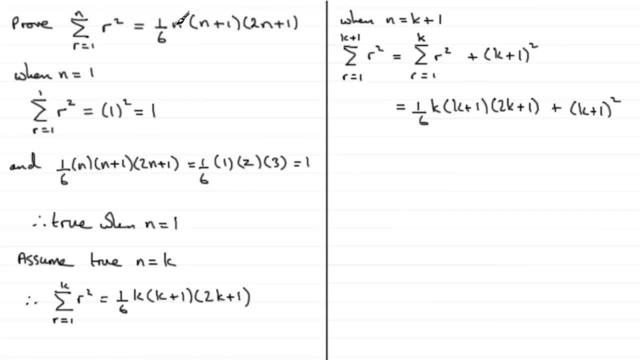 We're going to end up with all the n's being a k plus 1, and I can see that if I'm to do that, it'd be a good idea to spot that one sixth, and k plus 1 is a factor that is common to both this. 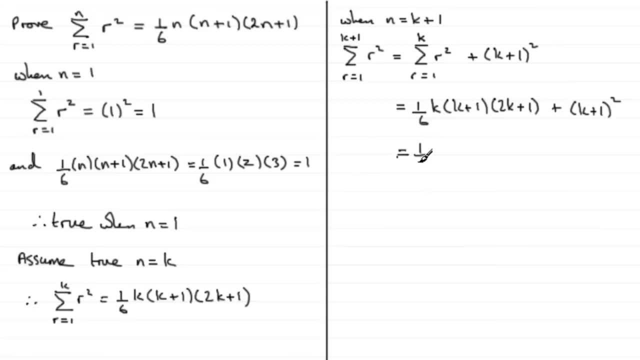 term and this term here. So I'm going to pull out one sixth k plus 1.. So that's looking quite good so far. I'm expecting to get in these two brackets, instead of n here, k plus 1 plus another one, and then two lots of k plus 1 plus that one there. 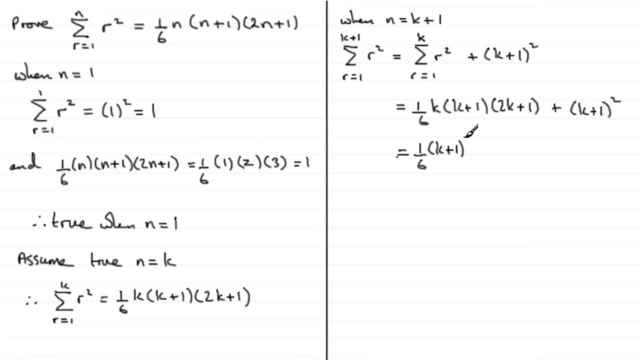 So it's given me clues all the way. So if I put up a square bracket here, what have we got to put in here now to get this first term? Well, it's got to be the k and the 2k plus 1, so we'll put k. 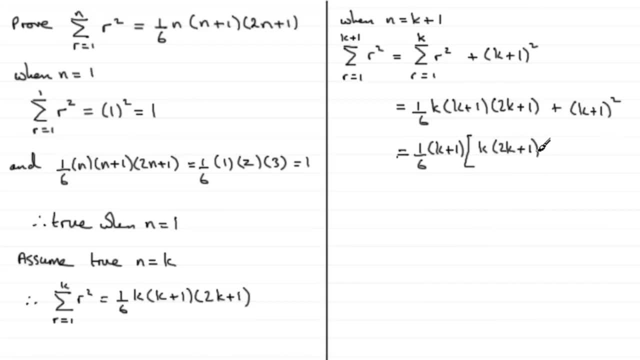 bracket 2k plus 1, and for the last bracket we've already pulled out one sixth, so we've got to make this six times bigger. so we've got plus six and we've also pulled out a k plus 1.. So we'll just reduce that down to k plus 1 there. okay, Now all we need to do is to just clean up. 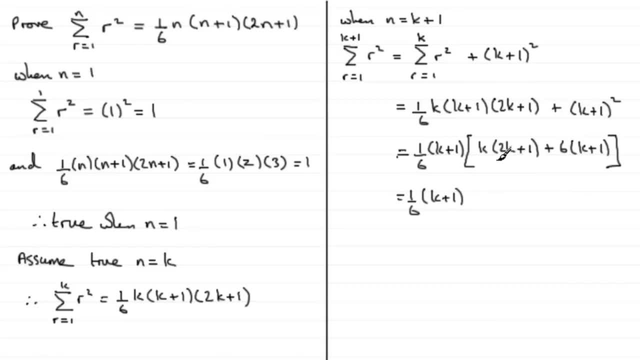 this square bracket here. So if we multiply this out, can you see we've got 2k squared, so let's just put that in as 2k squared. We've got k times 1, that's a k plus this 6k, so that's going to be. 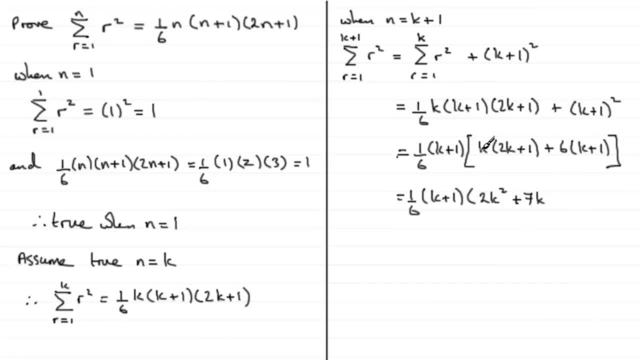 7k, and then we've got the 6 times the 1 on the end, so that's just going to be plus 6.. Now I can try and factorise this quadratic factor. We've got then 1 sixth k plus 1, and if we 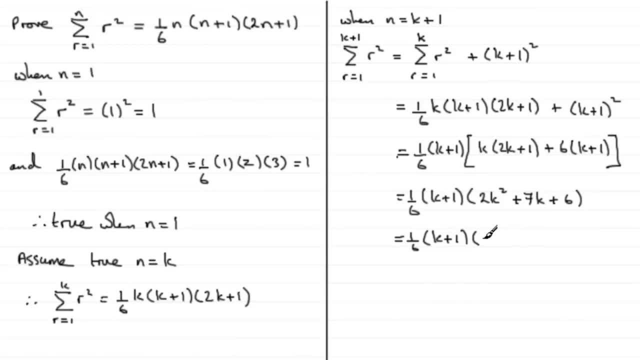 factorise the quadratic factor, you get two factors. One of them is 2k plus 3 and the other factor is k plus 2.. check that out, you'll see that you get the quadratic there now. I prefer to rewrite this now so you can see that we get this kind of format. 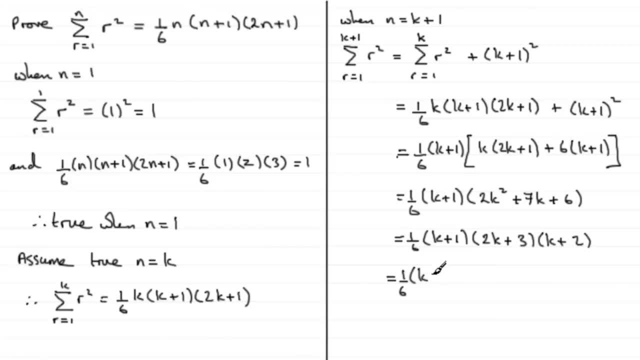 I get this then as 1 sixth k plus 1 now, instead of the k plus 2, I'm going to write that first of all. as we'll put it in square brackets as well, k plus 2 can be written as k plus 1 plus another one. so 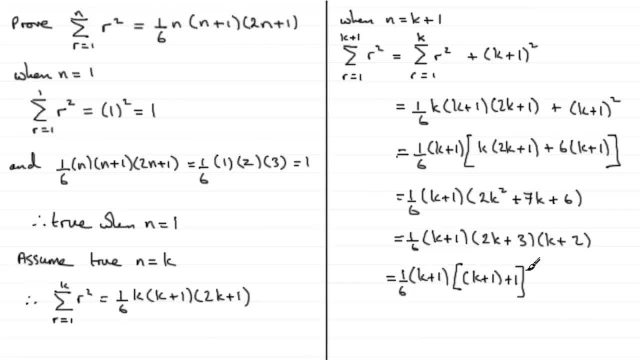 that's looking good for this bracket here. and then we're multiplying this- another square bracket there- by 2k plus 3, but we could see this as two lots of k plus 1 plus another one, so you can see that we've got the form 2. 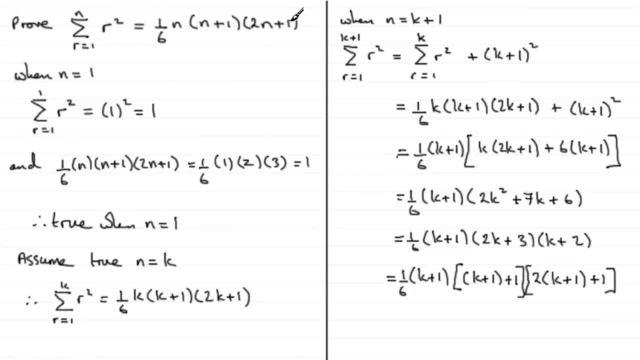 multiplied by k plus 1, and then the plus 1 on the end. so you can see it's true for. therefore, true for n equals k plus 1, and then we just need to finalize this in the usual way. we know that if it's true for.